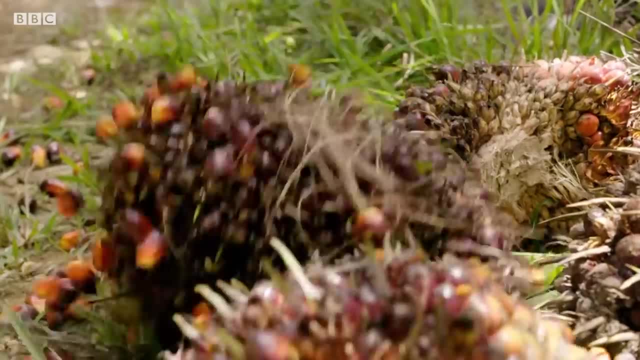 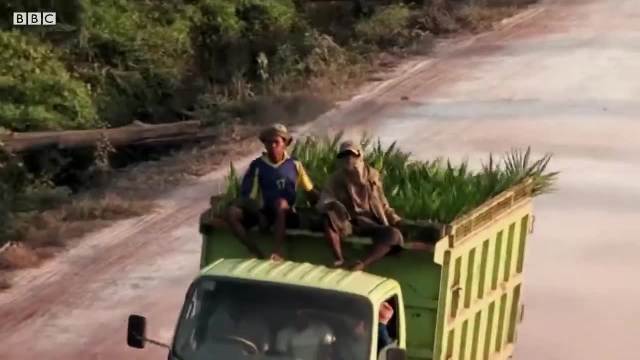 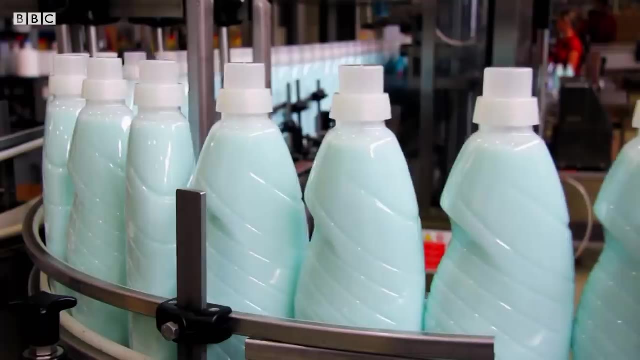 But one of the big drivers is palm oil. Palm oil is like a magical fruit. We all have palm oil in our houses right now. It's found in almost every good you can think about: It's in soaps, it's in shampoo, it's in chocolate, it's in bread, it's even in crisps. 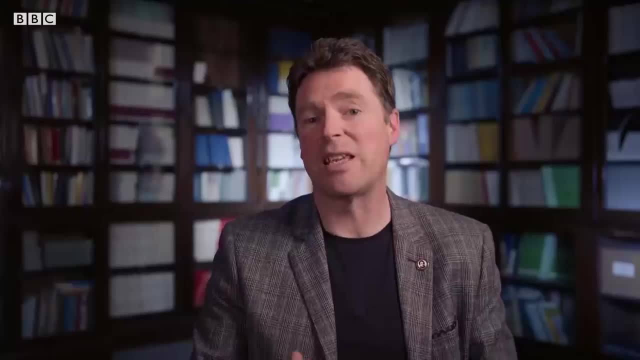 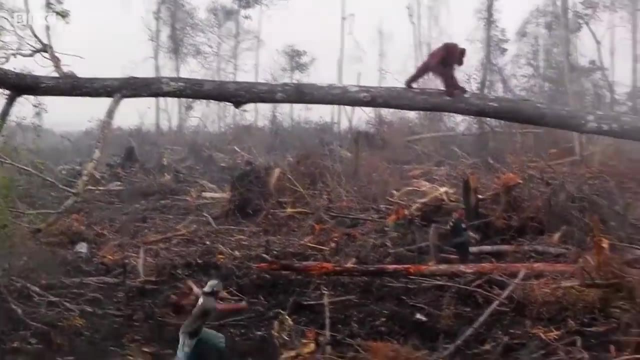 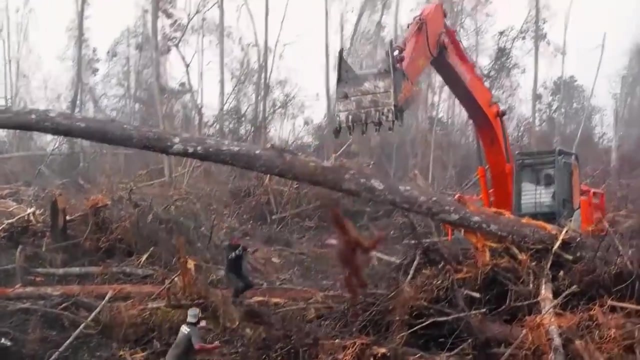 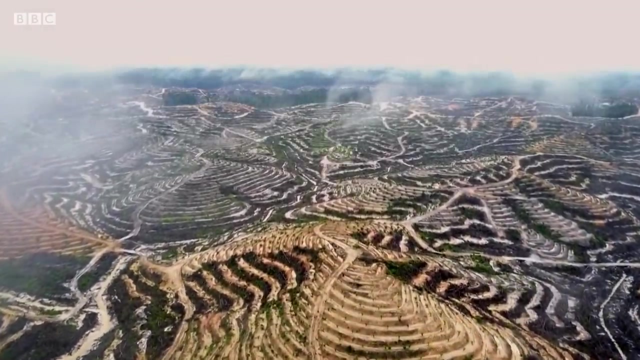 What we're doing, accidentally and inadvertently, is actually causing deforestation in other countries because our demand for this product. That means the natural system is not working, Habitats are disappearing, But also when these high carbon stock forests that are centuries old are cleared and burned. 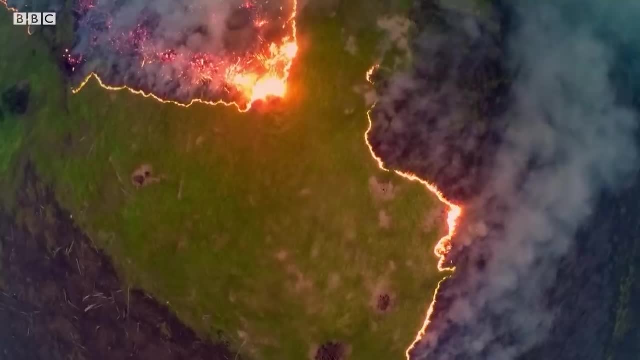 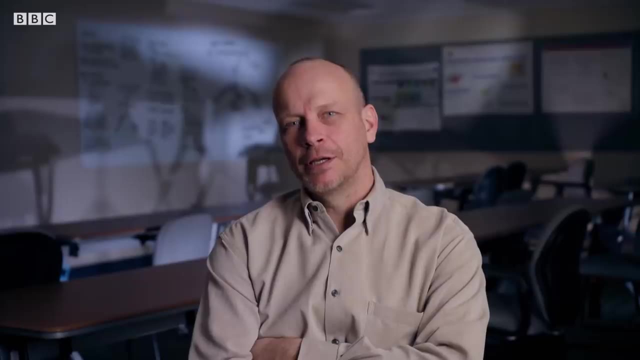 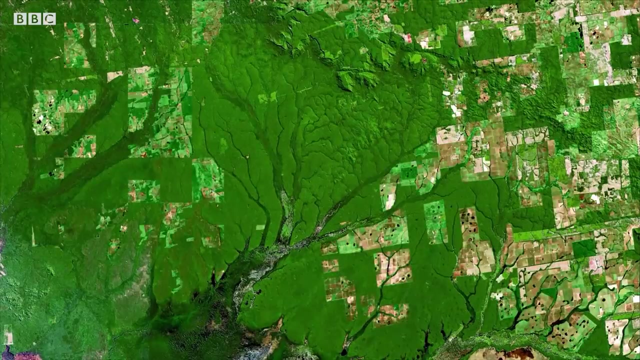 CO2 is added to the atmosphere. Those emissions go up and warm the planet. When you look at our maps, our results are showing that it's accelerating. It almost looks like a contagion, You know. it looks like a disease across the planet. 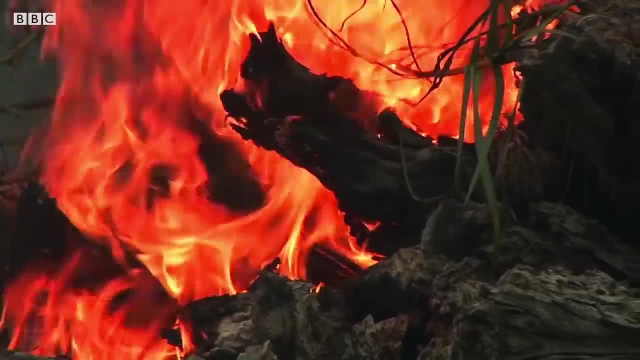 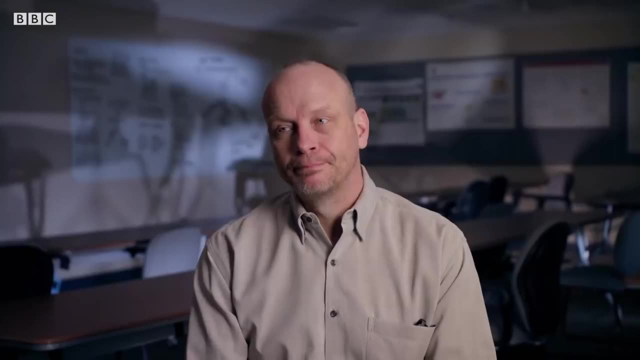 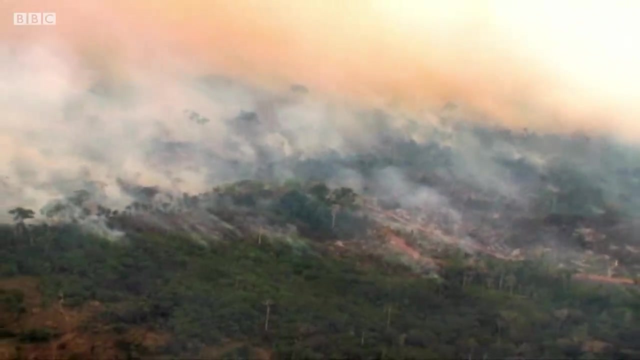 I mean the ever-increasing pattern. If we continue this level of deforestation, we'll take it all. Boom, there goes the forest, And our ability to mitigate climate change and turn the story around becomes really vanishingly small. But all of this is happening in the direction of the climate change. 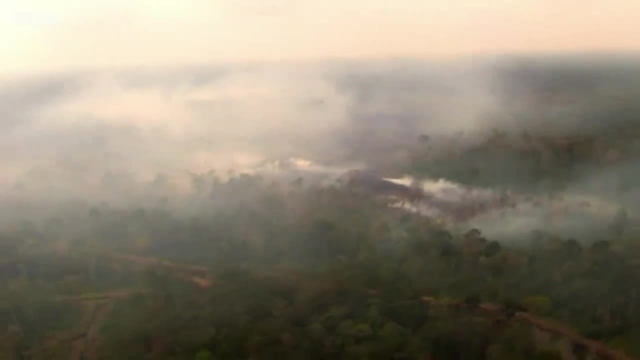 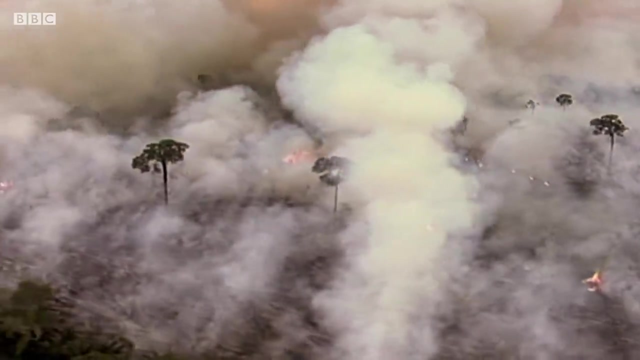 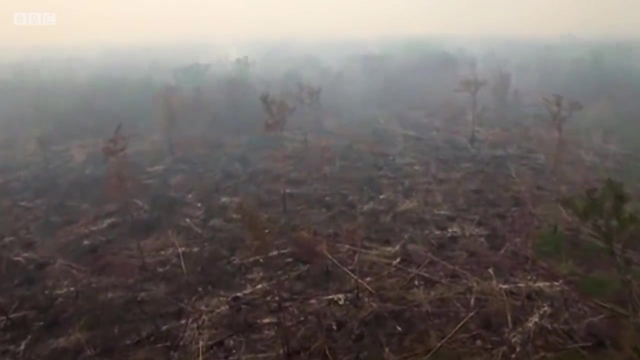 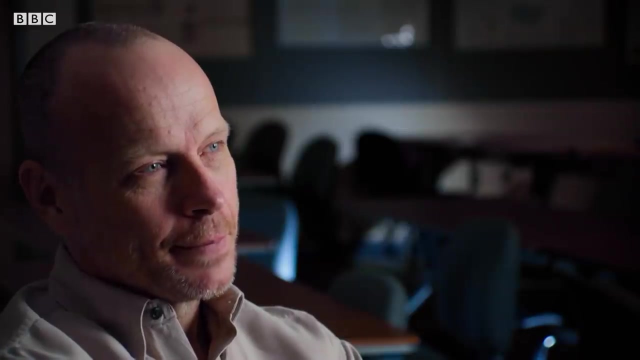 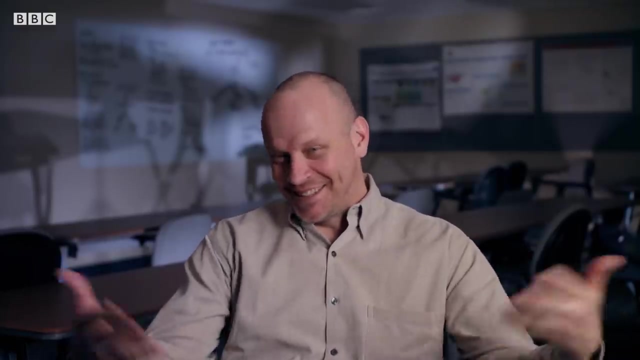 which is the most important thing, Trees are now being cut down and burnt at such a rate that nearly a third of carbon dioxide emissions are caused by deforestation. it sucks. I'm a pretty light hearted, optimistic guy, but just looking at these data, just looking at the stories, 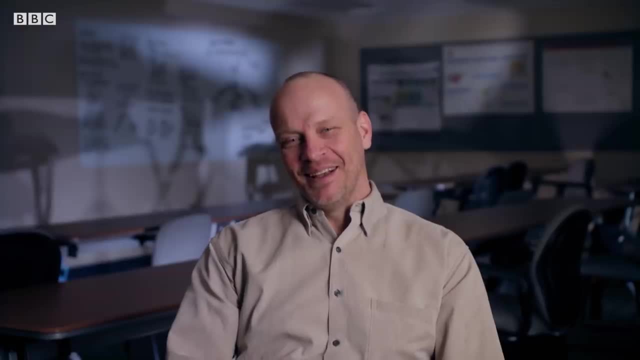 it's like I'd like to see some evidence of really strong kind of unified political response that was more than an aspiration on a kind of piece of paper right, That would be cool.